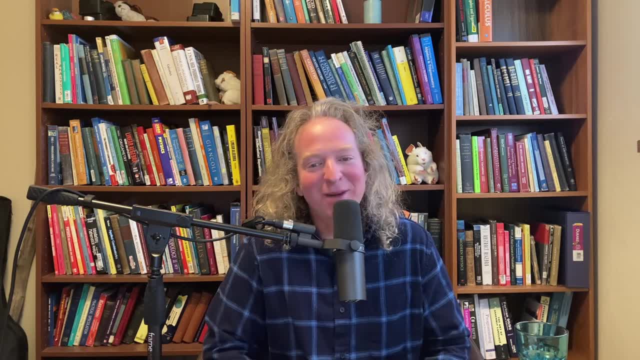 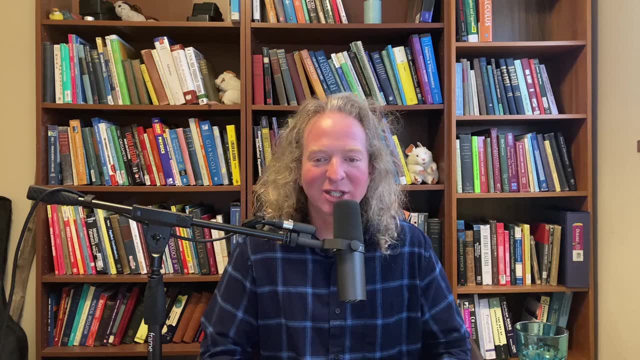 Okay, Hi, I am interested in studying mathematical statistics and I was wondering if taking your four Udemy courses, from Calc 1 to Calc 3 and Calculus, Integration and Sanity, would allow me to conquer a book such as Wackerly's Mathematical Statistics with Applications. Thanks a lot. 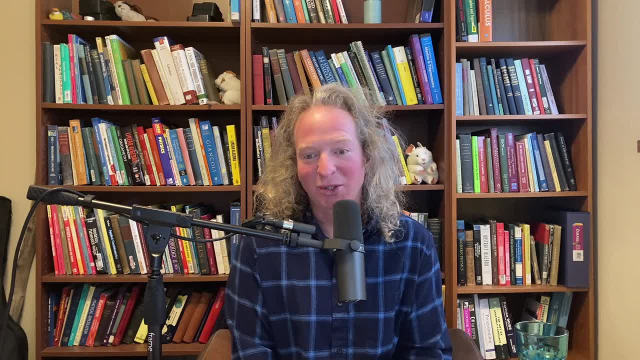 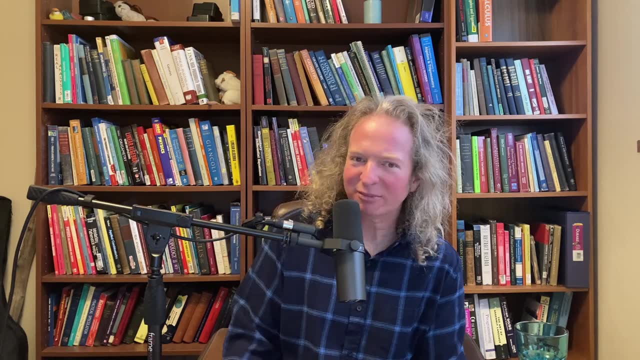 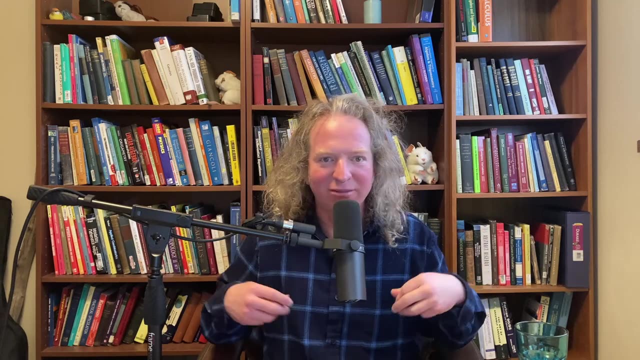 Okay, so that is a very interesting book. So the book he's talking about is called Mathematical Statistics with Applications and it's by Wackerly Mendel Hall and another author And it's a thick book. It's really thick And it's not like some amazing book, Like it doesn't read like you know an amazing book, It just reads like a math book. It's just a regular math book. 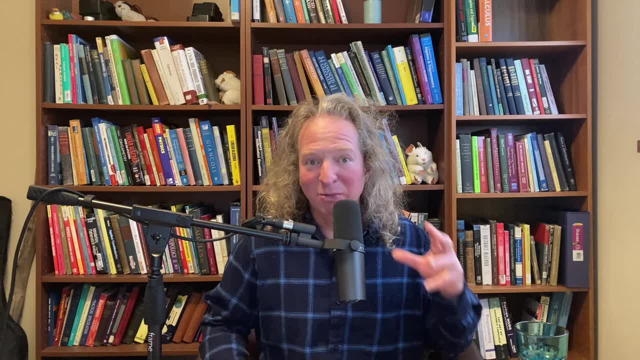 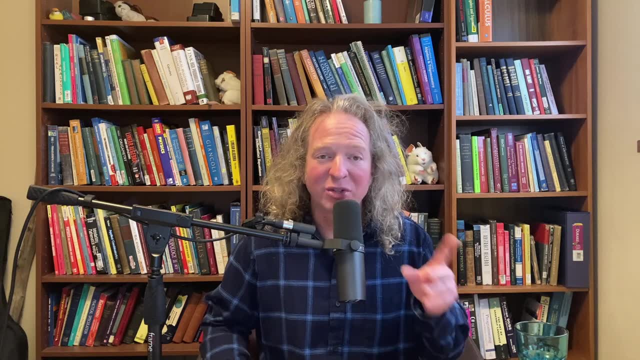 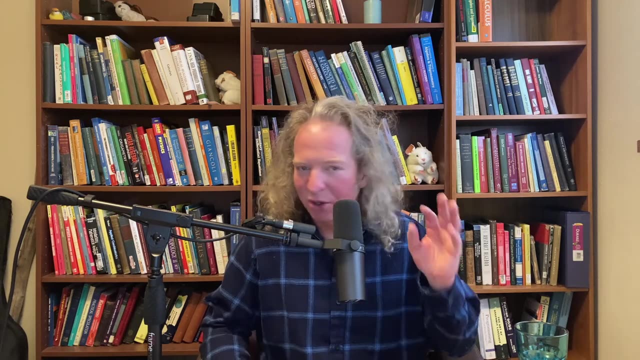 So what makes it special is that it covers so much material. Like, I have a couple mathematical statistics books and I feel like that one covers the material and it covers it well. Also, you can get a student solutions manual for that book. So my advice, Rowan, would be: just jump into it. Sure, you should take my courses. Obviously, I want you to buy my courses. 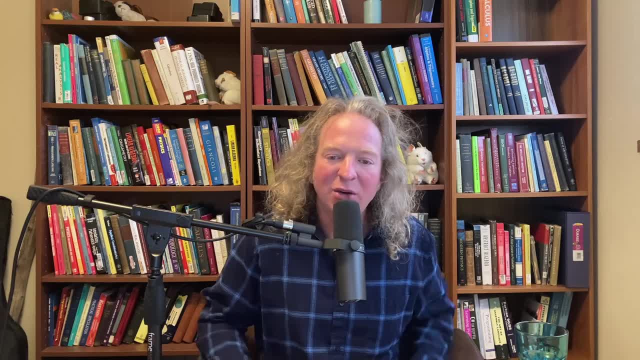 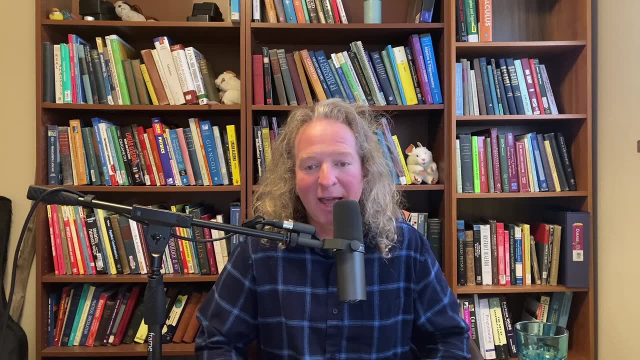 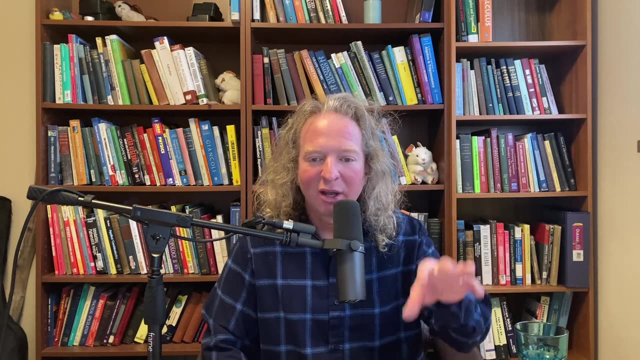 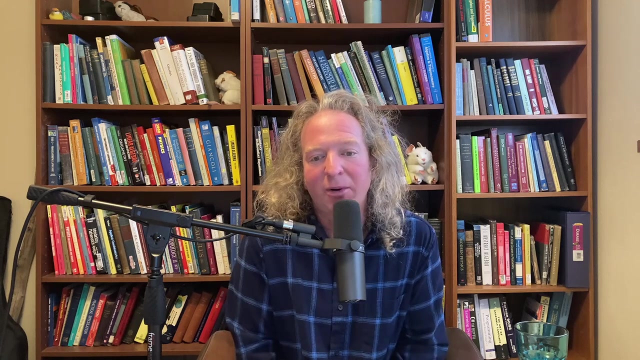 But honestly, you can just jump into it. You're not going to really see any calculus until you get later on to the book with some of the continuous distributions and stuff. And I actually have videos. I have a playlist that shows you how to do the calculus for those problems And the problems are actually from that book. So I've actually worked out some of the calculus-based statistics problems from that book. 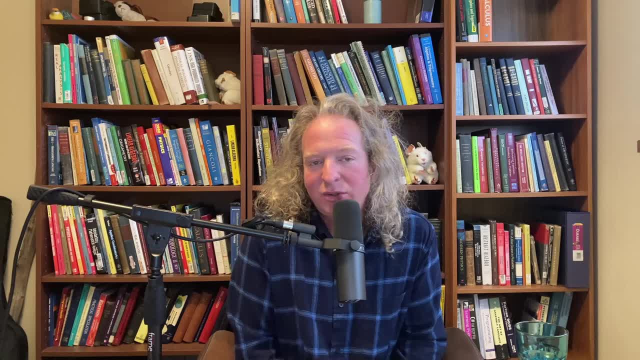 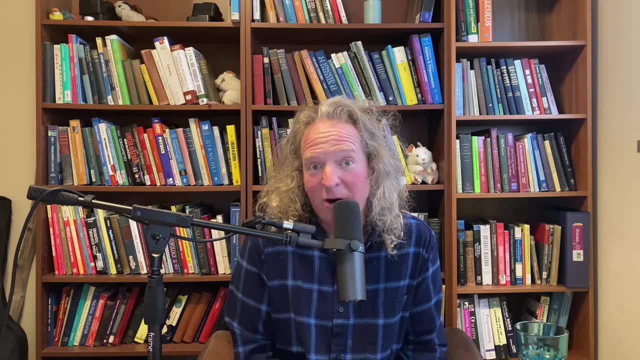 So I think you should just jump into it and see how you do. It's a hard book. My advice is: don't be discouraged. It's a very hard book. It's a rigorous book. It has proofs. It's a mathematical statistics book. 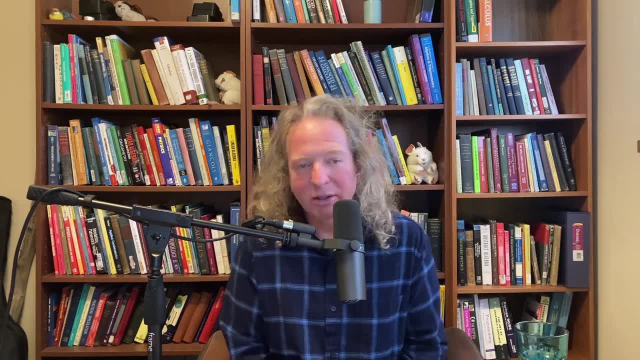 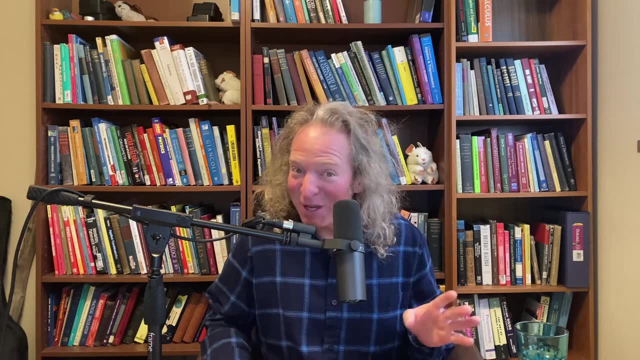 So that's my advice: Just jump into it And when the calculus comes up, then go back and review it. So I think it's cool you're jumping into statistics. Most people- I mean most people- there's a lot of people that don't like statistics. 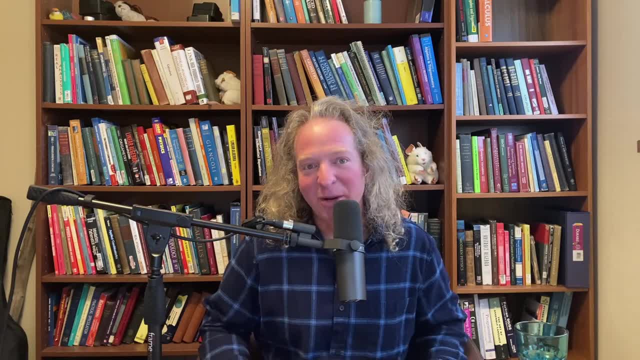 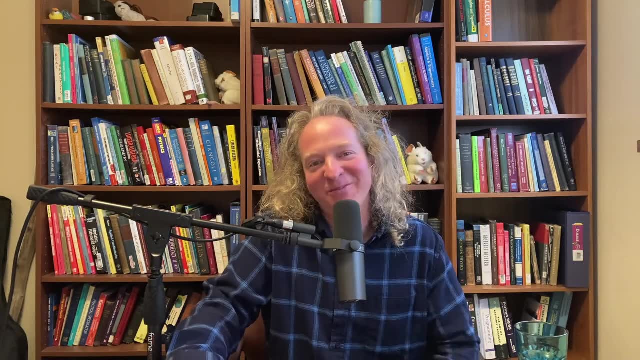 So yeah, I say go for it, Just jump into it and see how far you can get. If anyone else has any advice for Rowan, please leave a comment in the comment section below. Good luck.